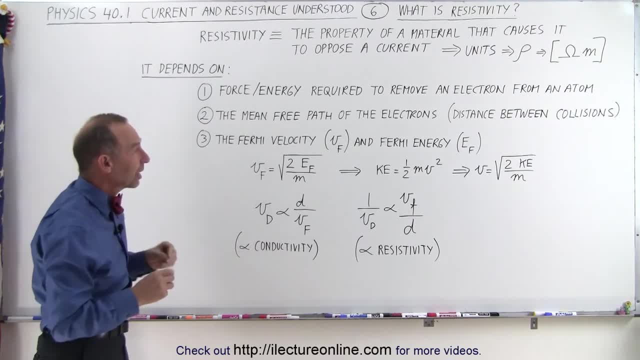 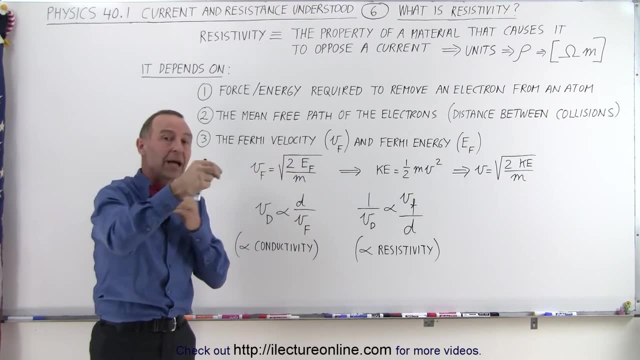 one of the main reasons it's called the mean free pad of the electrons. once the electrons are ripped free from the atom, they can move from atom to atom. well, they'll move a certain distance before they collide with another electron or with an atom or a set of electrons there, and so the distance 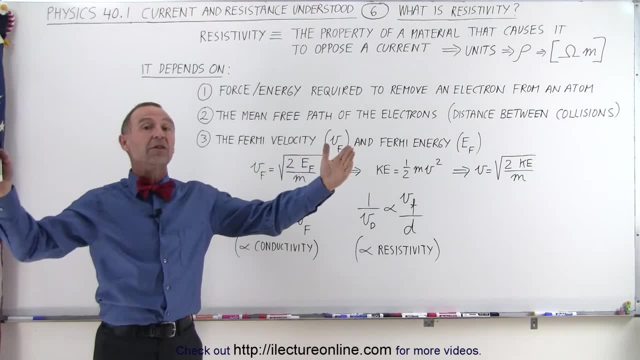 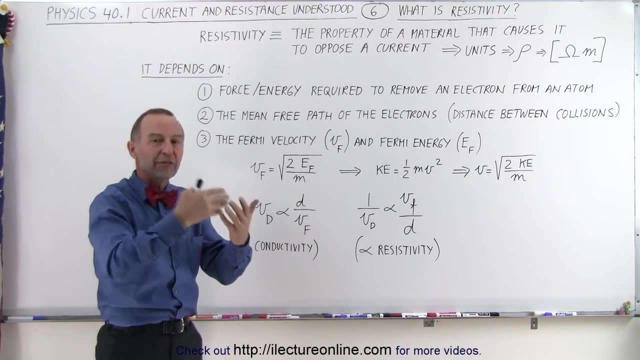 between those collisions is very important. the greater the distance, the more freely the electrons will flow. the smaller distance, the more often they will bump into something. the more difficult it is for electrons to flow through the circuit. so the resistivity is proportional to that. to that mean. 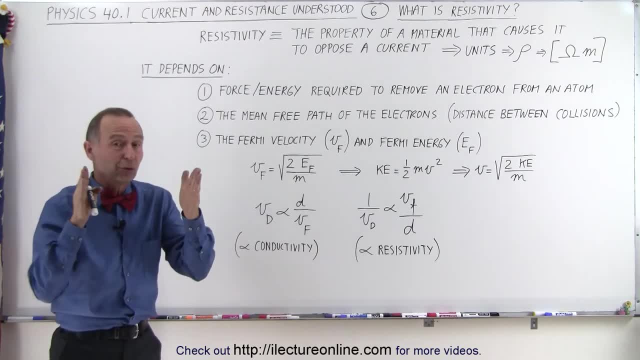 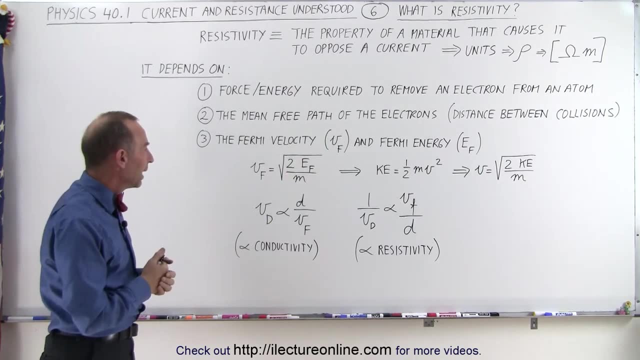 free pad, or actually i should say inversely proportional. the shorter the path, the greater the resistance. the longer the path, the less the resistance or resistivity. and it also depends on the fermi velocity and the fermi energy. well, the fermi velocity and energy will get into it a 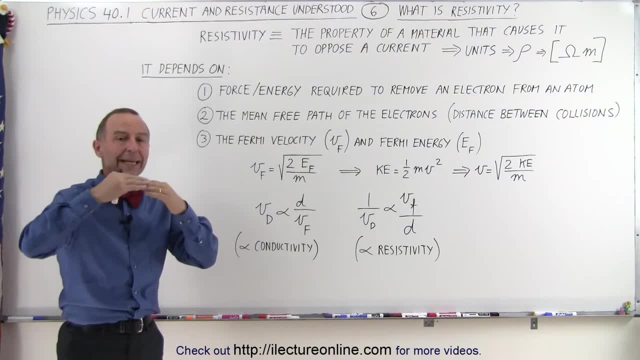 little bit more in a later video, but it has to do in. it has to do with the kinetic energy of Paulo Cant stories aboutNoir collision, and it has to do with the kinetic energy of the electrons or the particles inside a material at zero Kelvin and then the 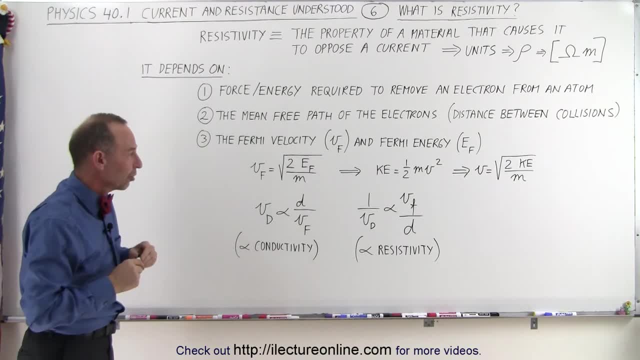 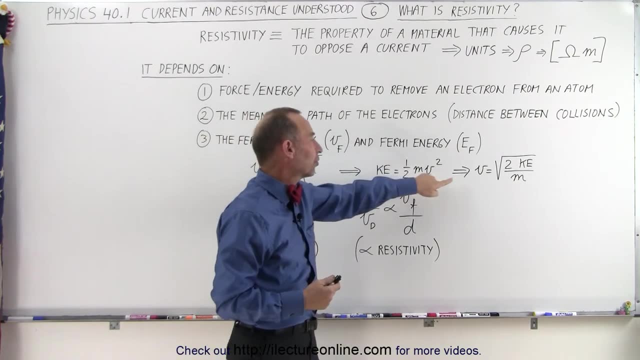 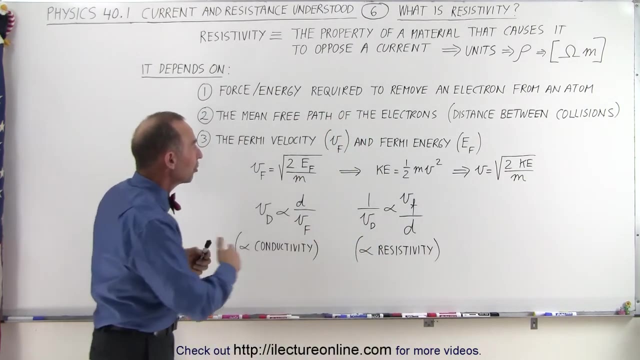 elevated energy need in order to move to the, to the material. so we remember that the kinetic energy of a particles one-half MV squared, so that the velocity is equal to the square root of twice the kinetic energy divided by the mass of the particle. there is a similar relationship between the Fermi velocity. 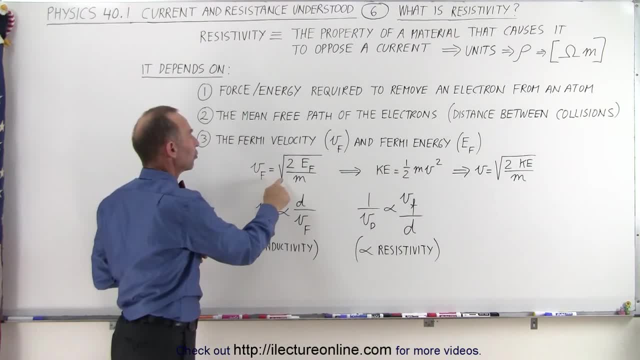 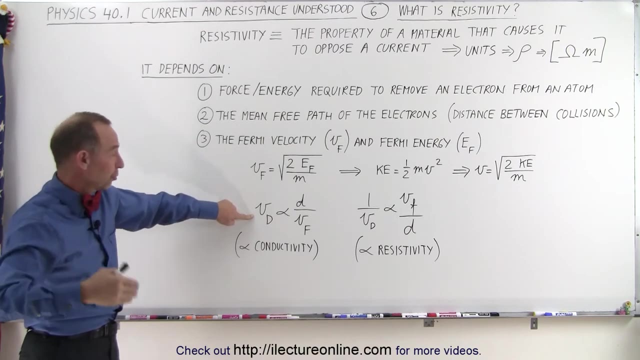 and the Fermi energy, in that the Fermi velocity is equal to the square root of twice the Fermi Fermi energy, which is basically kinetic energy of the particles divided by the mass. now, it's sufficient to understand at this point that the drift velocity, which of course is related to the current degraded the. 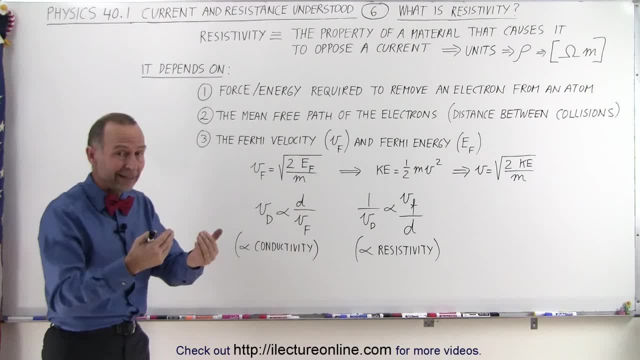 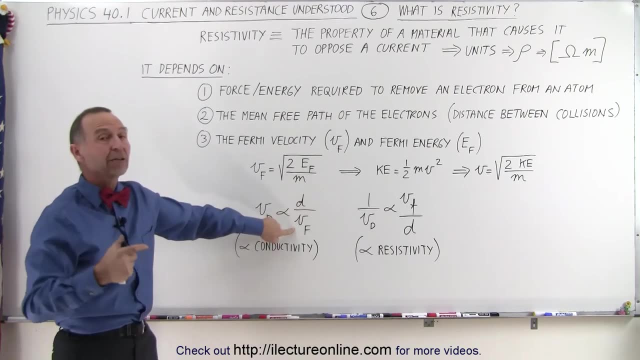 drift velocity, the greater the current. the smaller the drift velocity, the less the current. it's proportional to that distance between collision, the mean free path divided by the Fermi velocity. now, of course, the Fermi velocity is related and somewhat proportional to the Fermi velocity. 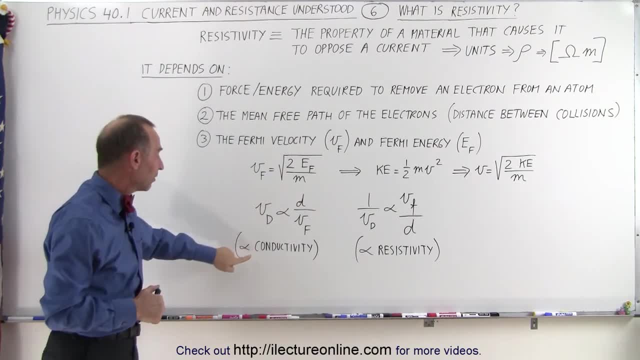 but here you can see that since the drift velocity is proportional to the conductivity, the freedom of the charges to move to the circuit is. therefore you can say that the greater the distance between collision, the greater the conductivity, and the greater the Fermi velocity, the smaller the conductivity or